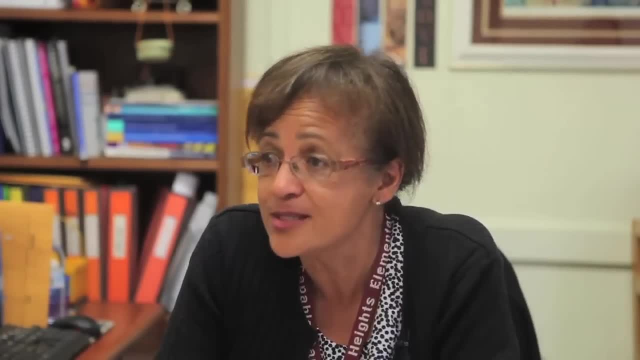 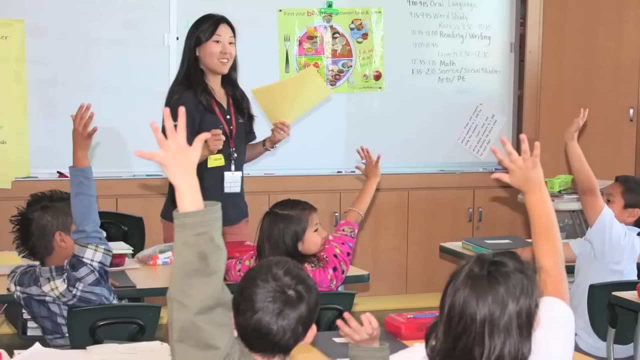 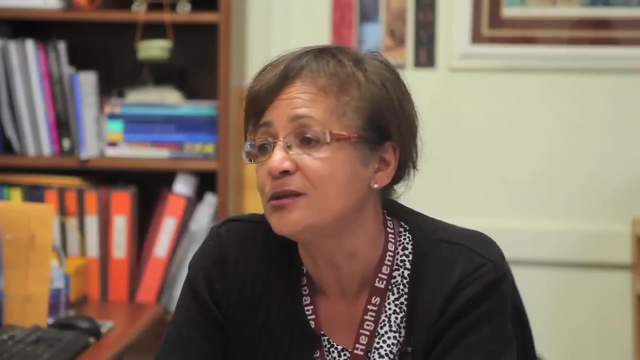 Well, I think it works because there's a really great staff from Cedars, the Healthy Habits folks who are really enthusiastic and creative And actually bringing in an example or working on a menu together with the classroom and for the children actually being able to see, touch and taste. you know, it makes it very real. 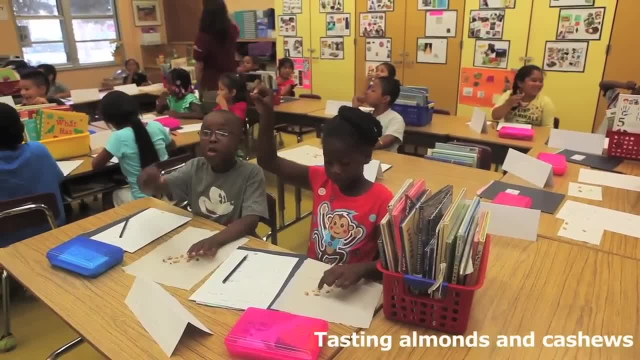 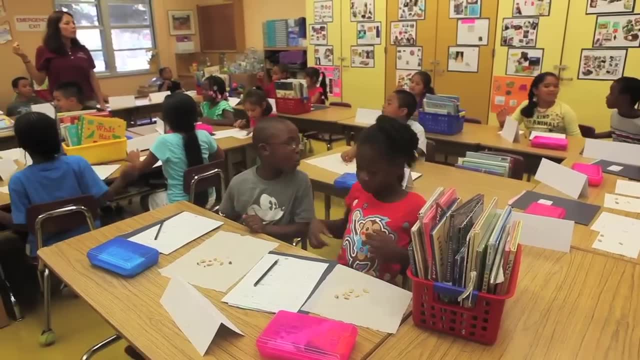 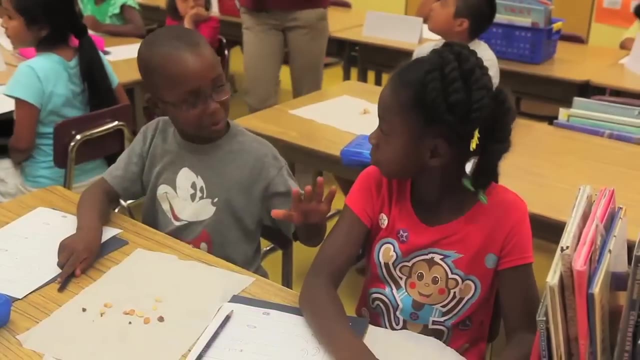 And you're going to put it in your mouth the whole thing, and you are going to try it, Ready On the count of three, Three, two, one Yum, I ate the whole thing. It tastes good, Good, yes. 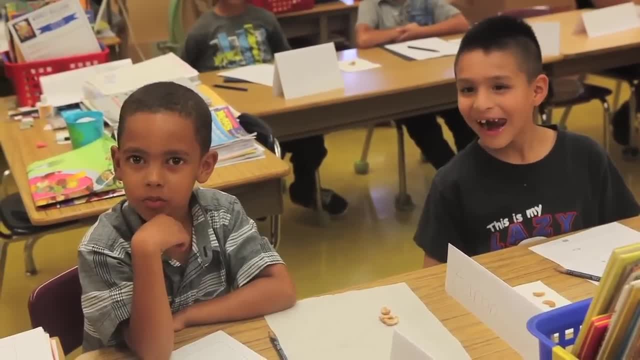 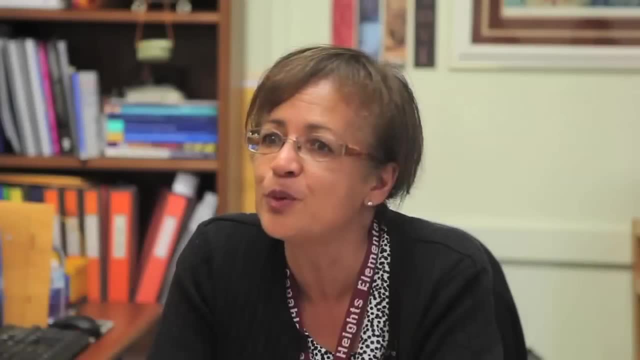 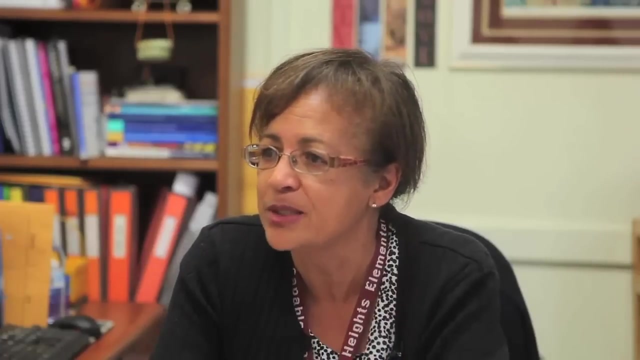 Did you like the almonds? They're sweet. They're sweet, Very good. I want some more, You want some more, And I think it's really important now because of the power of advertising and commercials. So then on television, you know, they're always getting bombarded with these messages. 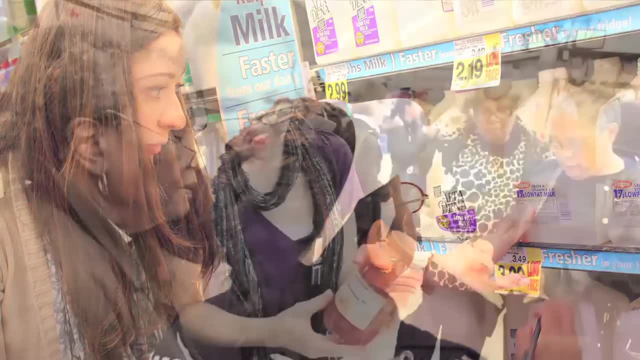 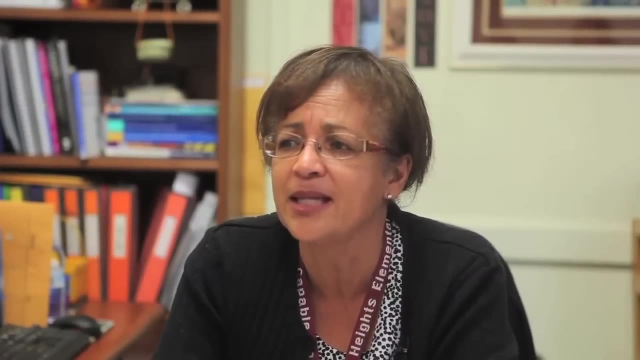 And I'm sure that when they go to the market you know it's like get this, get that. you know, And now hopefully You know, having that experience of being involved in the Healthy Habits class- they think about that a little bit more. 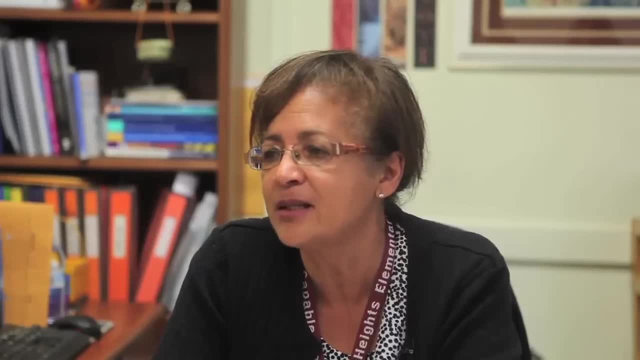 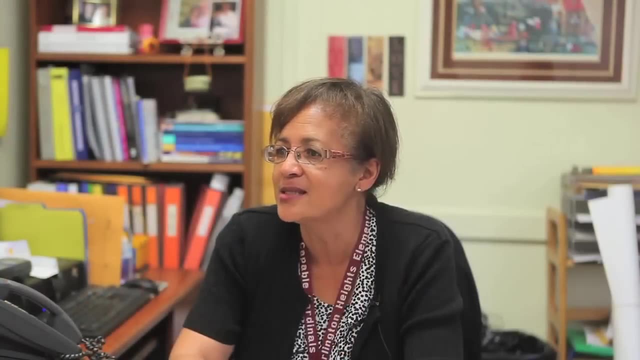 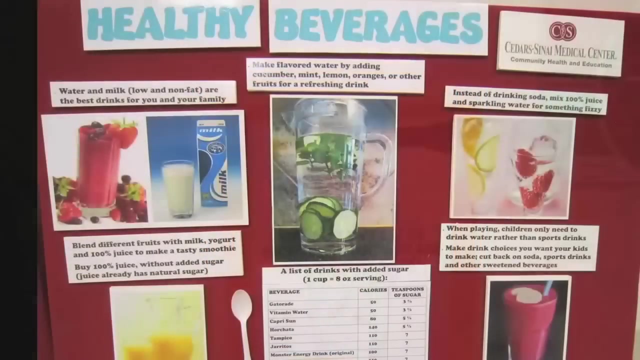 And I know with the teachers they have expanded our awareness or consciousness of how to read the labels and that sort of thing. During one of the teacher classes we got an idea of how much sugar is in like a soda or I think what kind of floored me was even in fruit drinks or Gatorade. 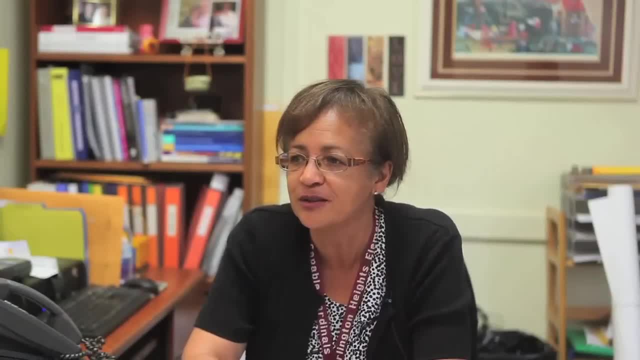 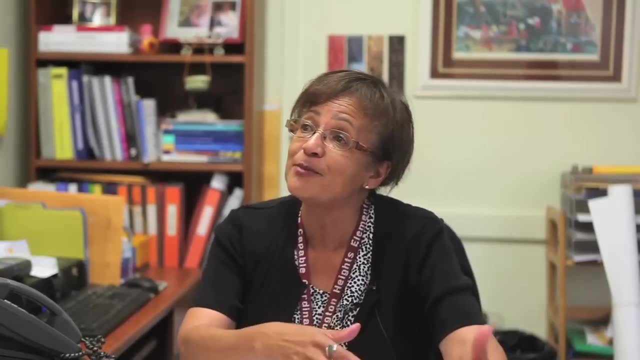 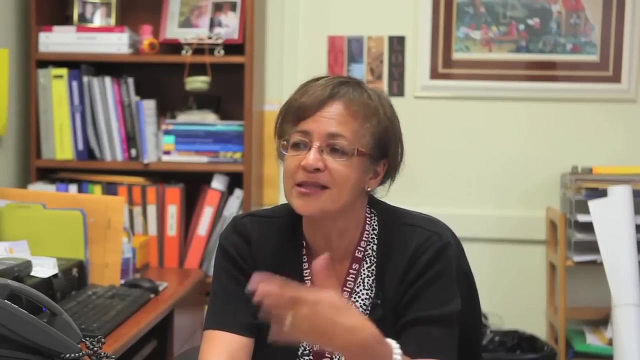 And as a result of that, you know I've pretty much given up sugar And I've also talked about that in the supermarket. So if somebody's within listening distance and I'm with somebody I'll say: did you know that if you read this and divide it by four, you'll know how many teaspoons of sugar you know is in that particular drink. 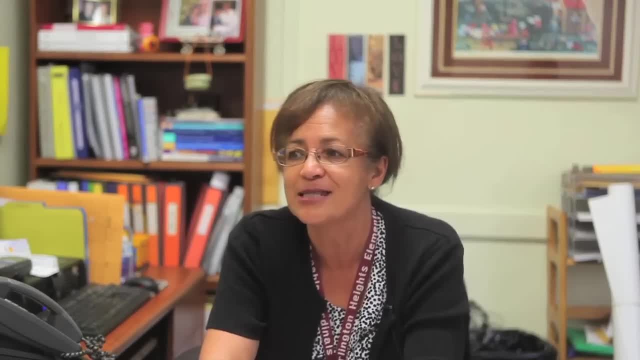 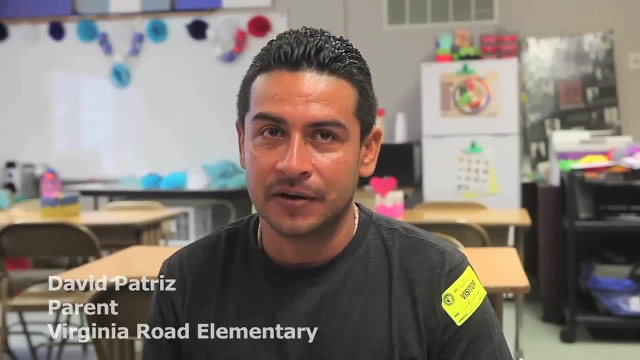 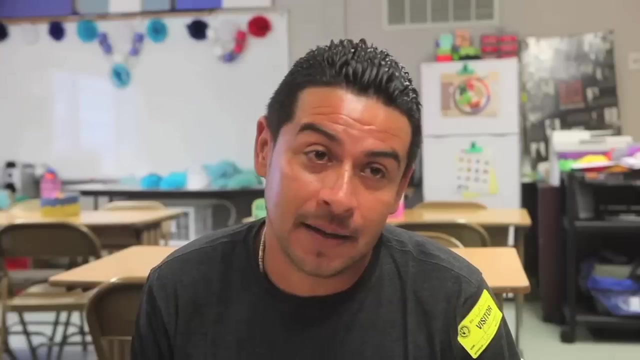 So I've become a Healthy Habits messenger. outside of school. The first thing I learned was not to drink soda anymore, because before I used to be a parent to buy a lot of soda and have my kids used to drinking soda. But ever since I came to this class I started not buying soda anymore and I just drink water and juices. 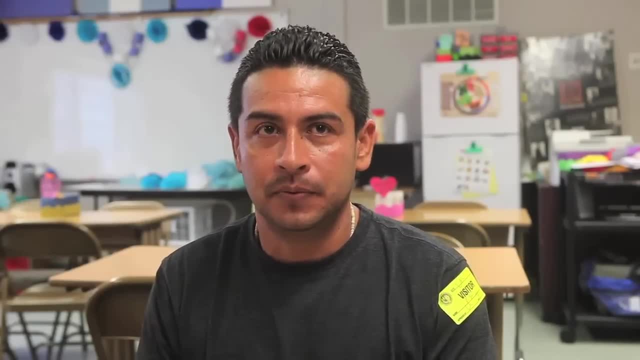 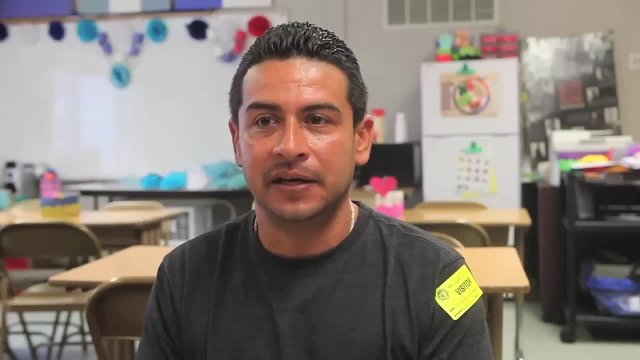 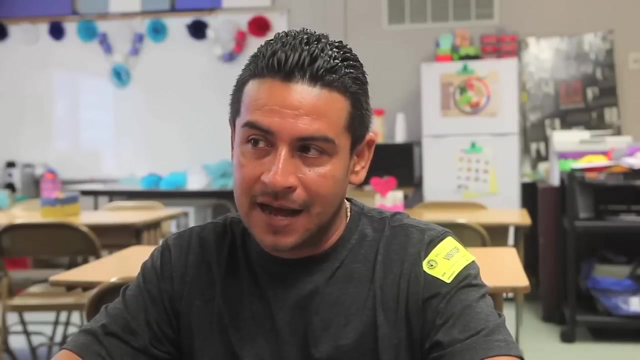 The other way I cook. I put more vegetables in my plate, try not to eat red meat as much, try to eat just chicken, fish and a lot of vegetables and fruits. Every time she says the Healthy Habits is going to come to our class, she gets really excited and happy. 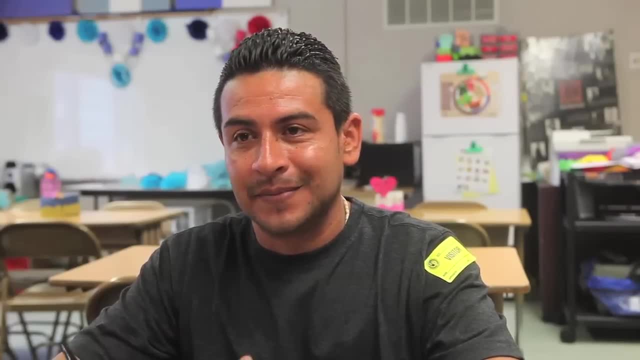 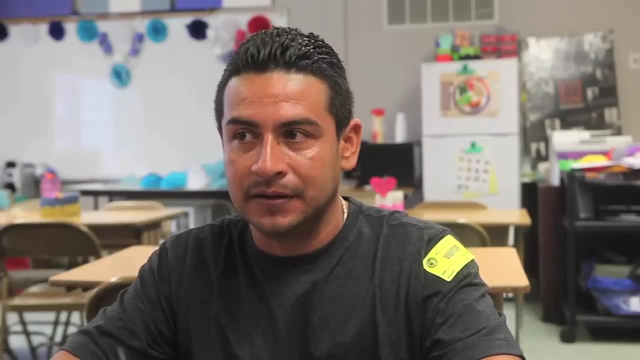 And she always tells me to do The recipes for how to do, like you know, the snacks that, instead of eating her snack when I get home she tells me: Dad, can you cook for me what they gave me at Healthy Habits? and try to do it. 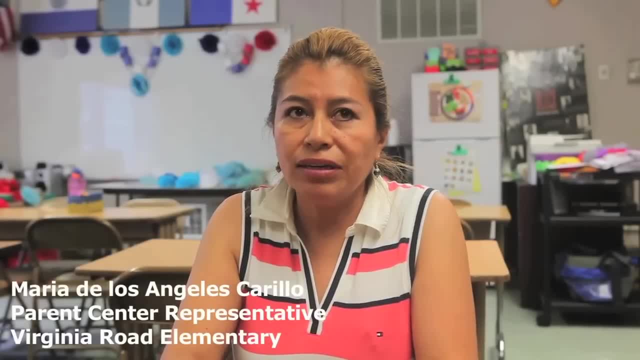 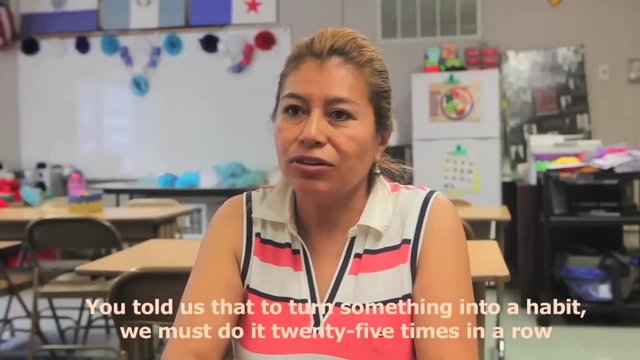 Pues sí, en mi familia sí, porque lo primero que hice y que tomé así bien en serio, fue lo de cómo hacer un hábito. Y pues usted nos enseñó que un hábito lo tenemos que hacer para que sea un hábito. 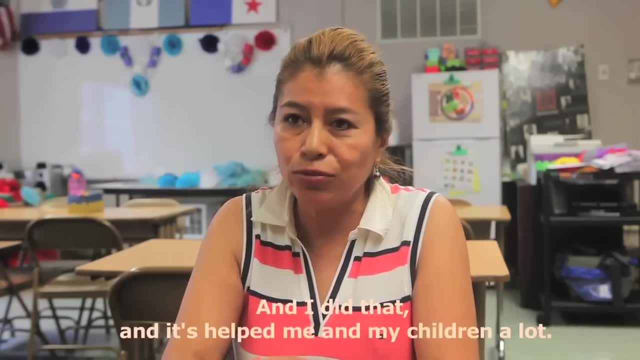 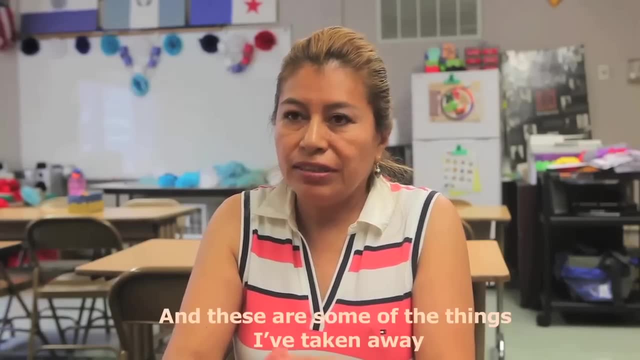 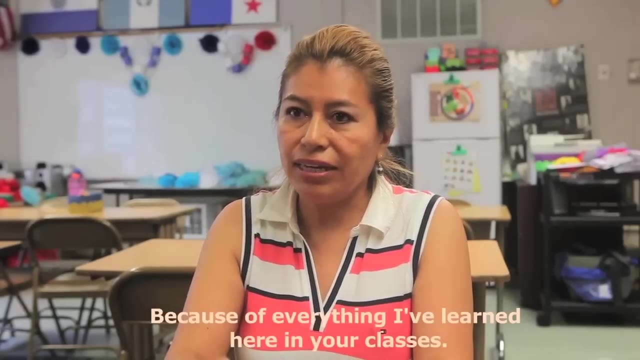 Veinticinco veces seguidas, Y eso lo hice y me ha funcionado mucho con mis hijos Y yo rebajé quince libras, casi veinte. bueno, Y pues son de las cosas que he tomado y más aparte, pues no tomo soda, no como mucha harina, porque todo lo he aprendido aquí en las clases de ustedes. 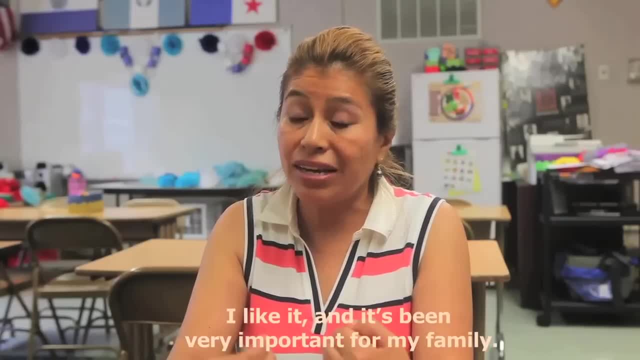 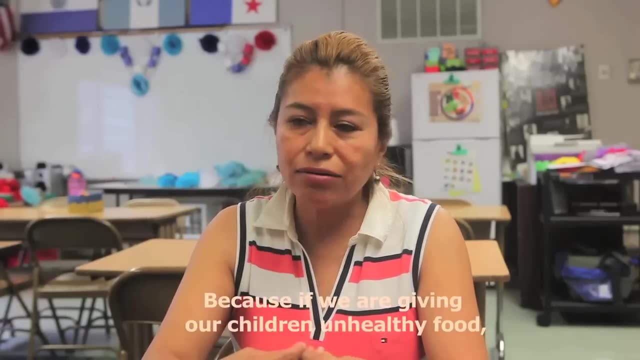 Entonces, pues, a mí me gusta esto y para mi familia ha sido muy importante, Entonces, pero yo pienso que eso es bien importante porque los niños, si nosotros les estamos dando comida no saludable, ellos nos recuerdan. 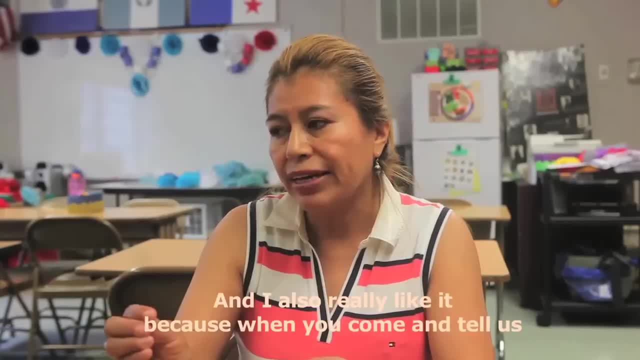 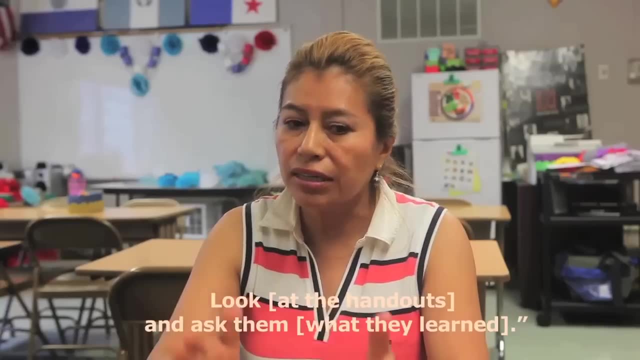 Entonces eso es bien importante y me gusta mucho también, porque cuando usted viene y les dice: los niños están también tomando la clase, vean, pregúntenles. Entonces es bien importante que tanto los niños como los papás lo estén viendo, porque si a nosotros se nos olvida, 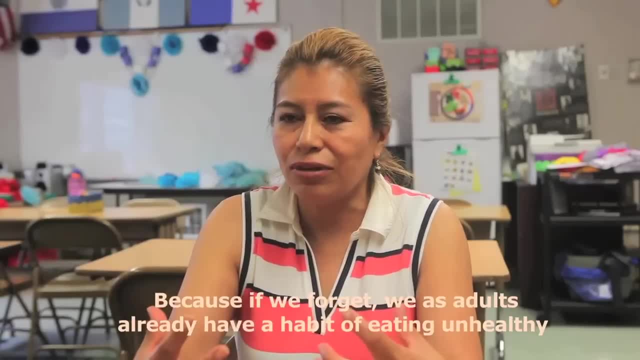 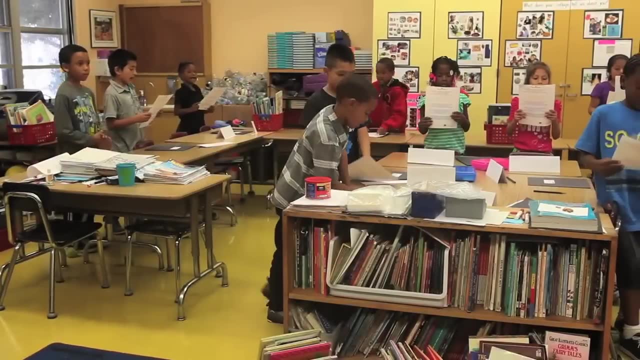 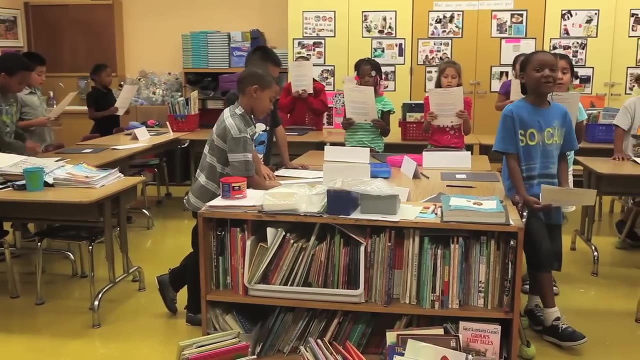 Porque nosotros, como adultos, ya tenemos una costumbre de comer no saludable. Y si ellos nos enseñan? oh qué vergüenza. Pero bueno, We practice healthy habits at home And school each day. Five basic food rules will make us strong and play. 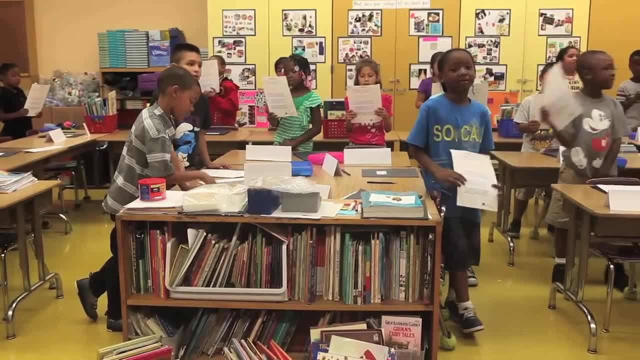 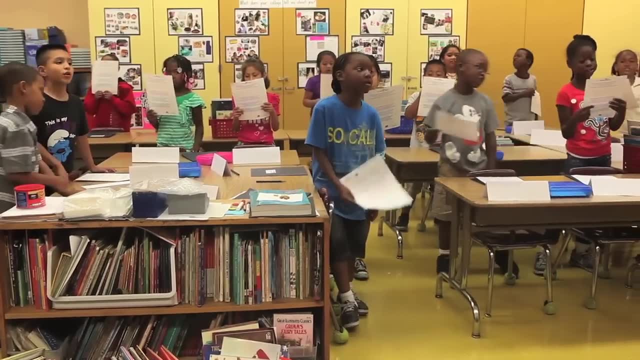 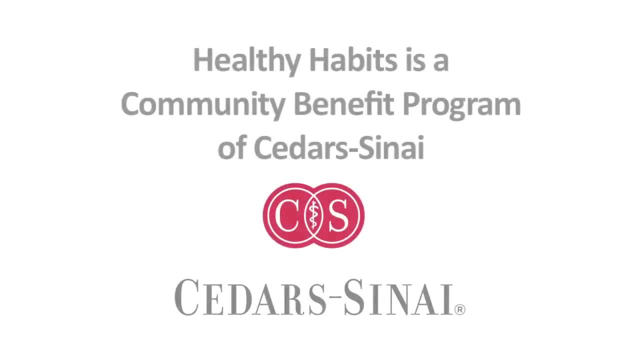 So many fruits and veggies to fill up half our plate, And they help us to be active and make us feel so great. We'll see you next time.